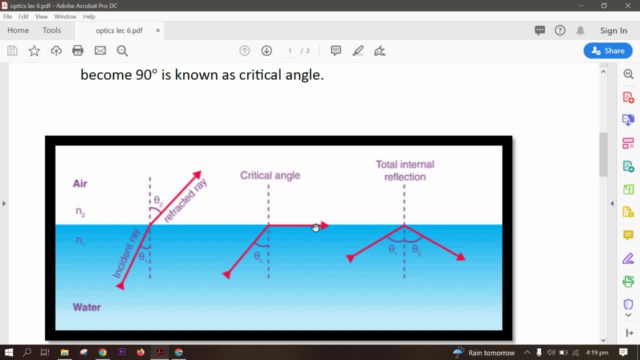 patting after light on light return, as light is outside light, the angle of creating a little undertaking. it will move straight on the change in medium boundary. it will move straight on that boundary, it will be parallel to that boundary and because of that it will be an angle. 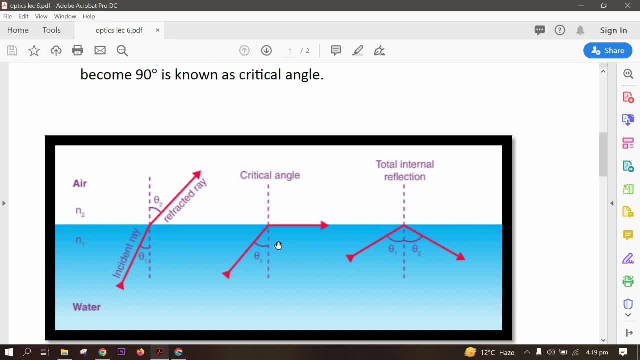 I have told you earlier that my angle of incidence and angle of refraction are being normal. so my normal will be angle of refraction with angle of refracted ray, and you can see that when angle of refraction will be made then it will be 90 degree. 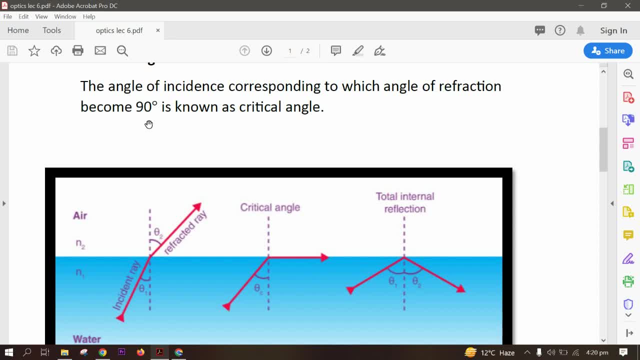 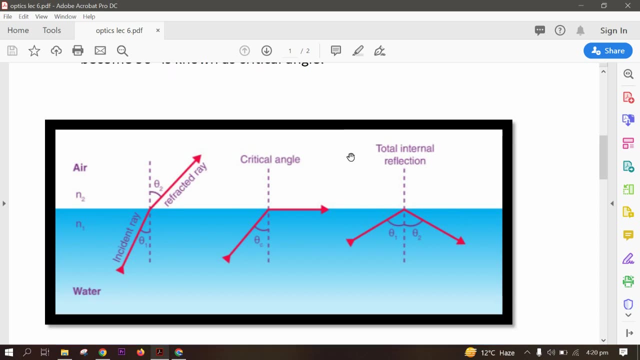 so this kind of angle of incidence, because of which angle of refraction will be 90 degree, that angle of incidence will be called critical angles. did you understand this much? ok, now the question is that how critical angles relate to total internal reflection. so, class, you have to remember this. 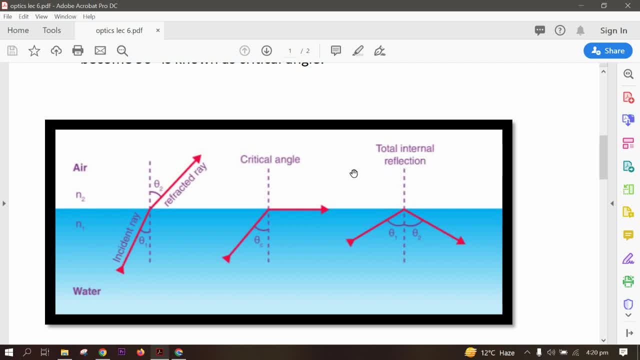 that when my angle of incidence will be less than if from critical angle, then my case of refraction will be regular refraction ok. and if my angle of incidence will be greater than critical angle, then if my angle of incidence will be greater than critical angle, then my incident light ray will not reflect in any other medium. 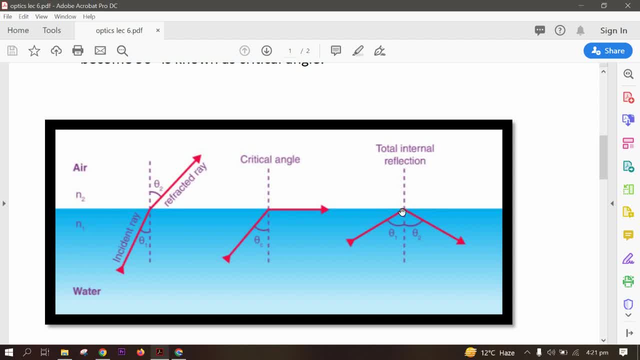 but it will bounce back in the same medium from which it is traveling. and I will tell this phenomenon what is this phenomenon? total internal reflection. you know, reflection is when light ray again bounce back in same medium. then I will tell this phenomenon that this is my total internal reflection phenomenon. 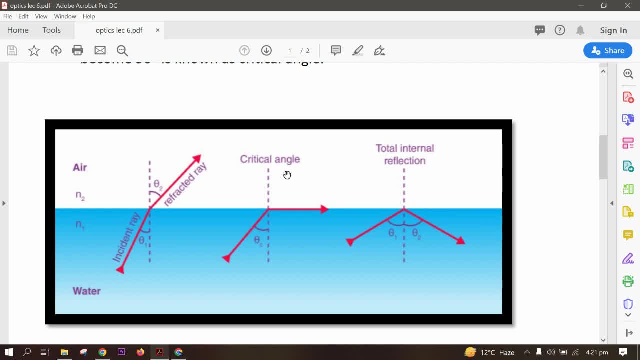 ok, class. you have to remember this: that when I talk about critical angle, then every material has its own critical angle. every material does not have only one critical angle. ok, we will discuss this in detail in the lecture of applications. ok, you can see on your screen the definition of total internal reflection. 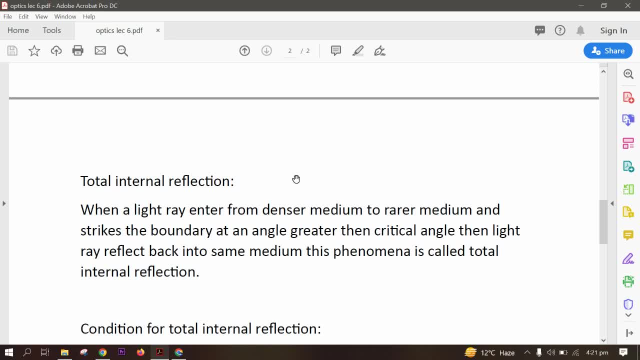 so that your concept will be more clear. what is written in that when a light ray enters from denser medium to rare medium. now what does it mean by denser medium? either I have a glass body or any water surface, or light ray is travelling in water. 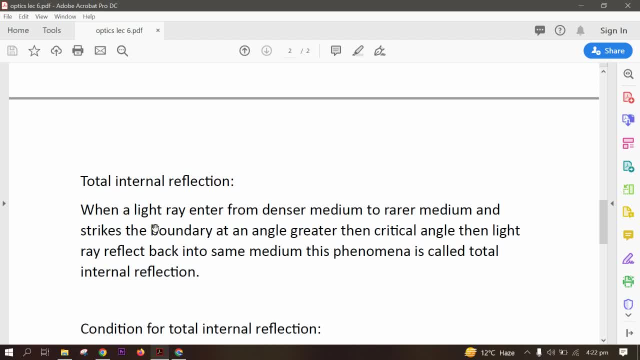 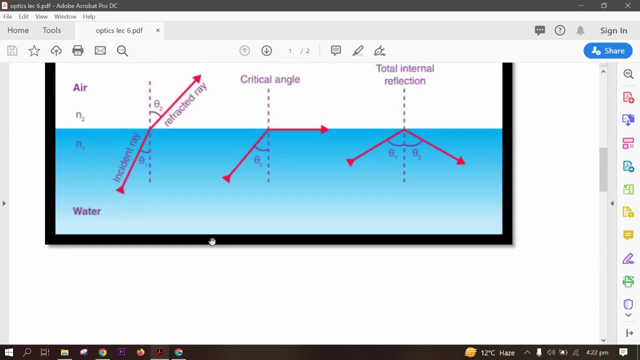 ok to rare medium and strike the boundary at an angle greater than critical angle, then light ray reflects back into same medium, which is denser medium. this phenomenon is called total internal reflection. ok, class, now you have understood that to observe reflection we have to have more angle of incidence. 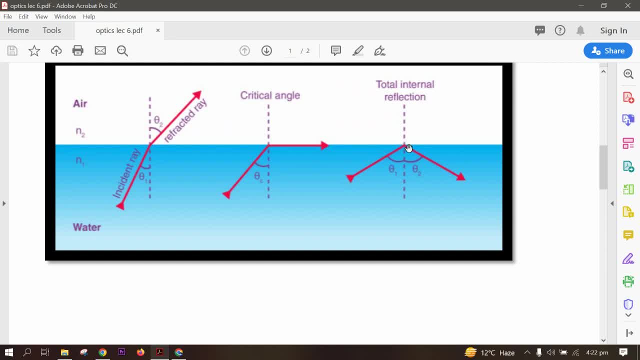 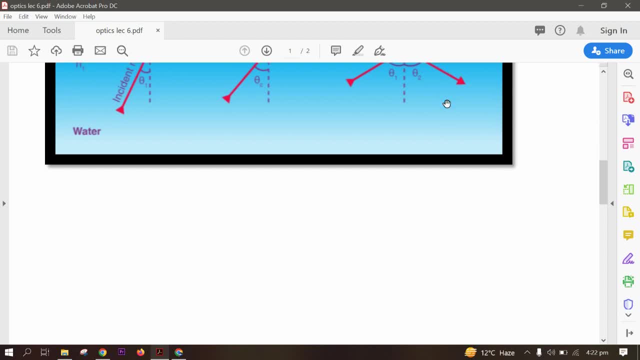 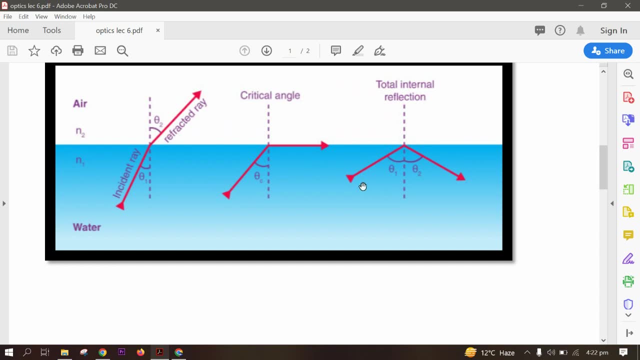 than critical angle after this class. on one more thing: total internal reflection depends on me, that is, my light ray basically travels from denser medium to rare medium, then only I will observe the phenomenon of total internal reflection, if my light ray does not travel from denser medium to rare medium. 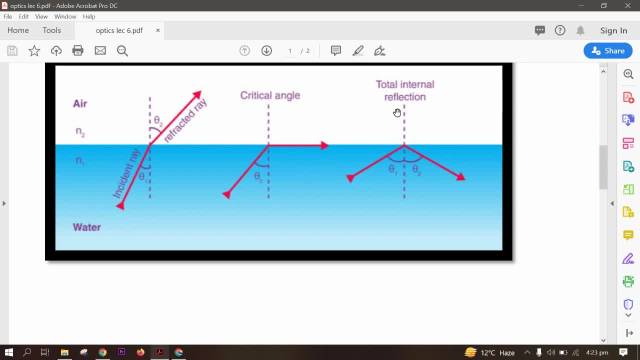 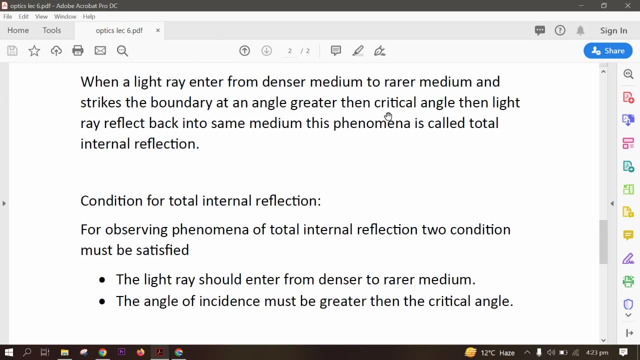 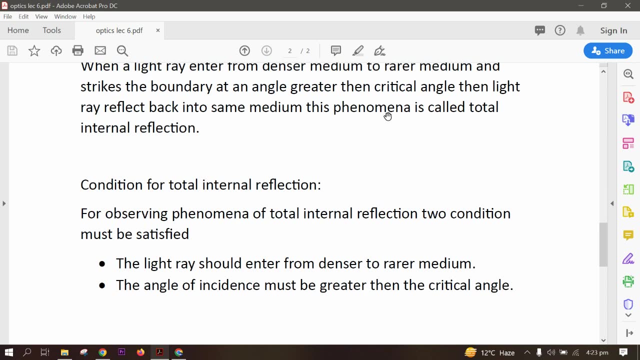 then I will not be able to observe the phenomenon of total internal reflection. ok, so I write that conditions for total internal reflection. for observing phenomena of total internal reflection, two conditions must be satisfied. first, my light ray enters from denser medium to rare medium, and second condition is: 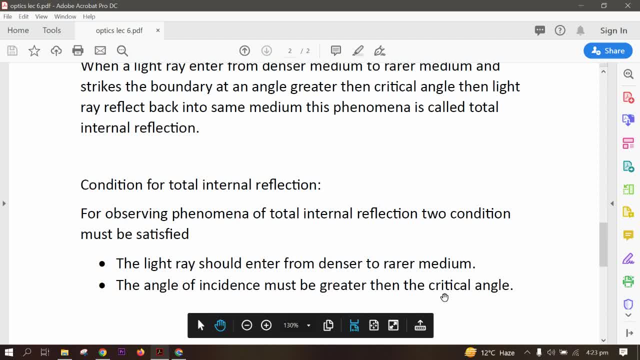 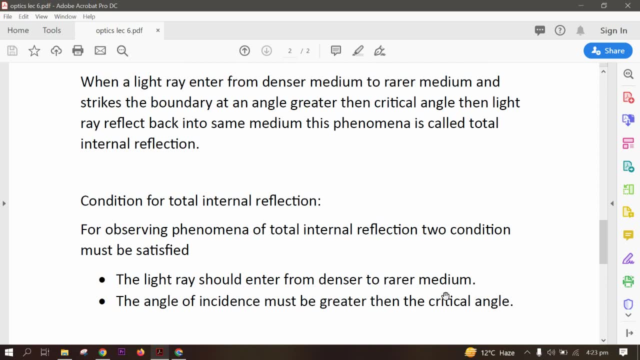 angle of incidence must be greater than the critical angle of material, because every material, of every medium, has its own critical angle, which we will see further in the topic of applications of total internal reflection in detail. ok class, I hope you have understood today's lecture, in case. 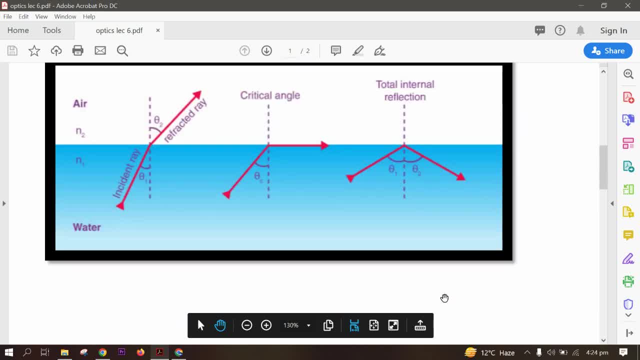 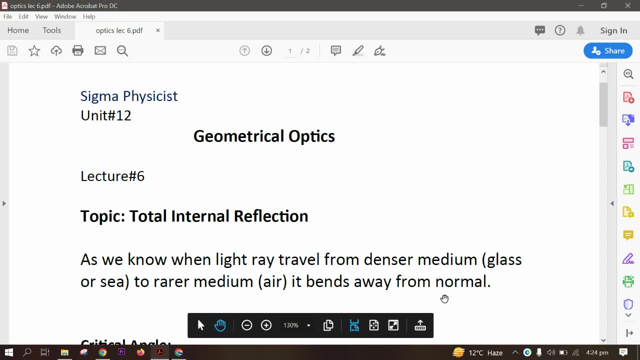 if you have any question, then you can ask in comment section and you can also DM me on Instagram. I will meet you in the next video lecture. till then, take care of yourself.